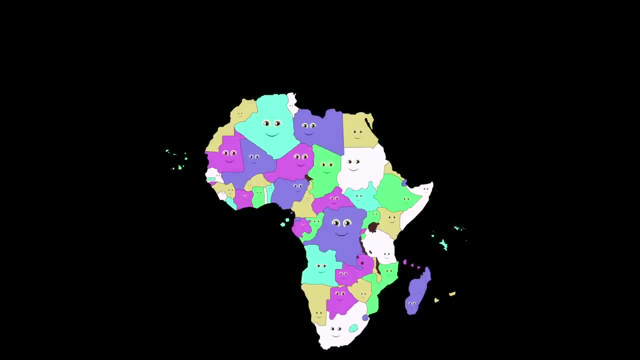 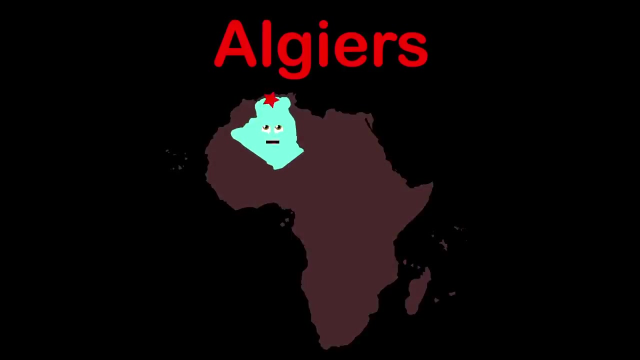 We are the countries of Africa, Our planet's second largest continent, right after Asia. We are the countries of Africa. There are 54 countries presently that we will teach you. My name's Algeria. My capital is Algiers. I'm Angola. Rwanda's been my capital for years. 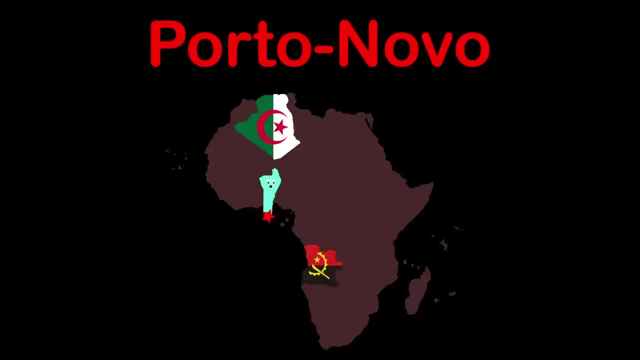 Benin is my name. My capital's Porto Novo, Botswana's my name. Gaborone's my capital. I'm Burkina Faso. Ouagadougou's my capital. My name's Burundi. Ujambura's my capital. 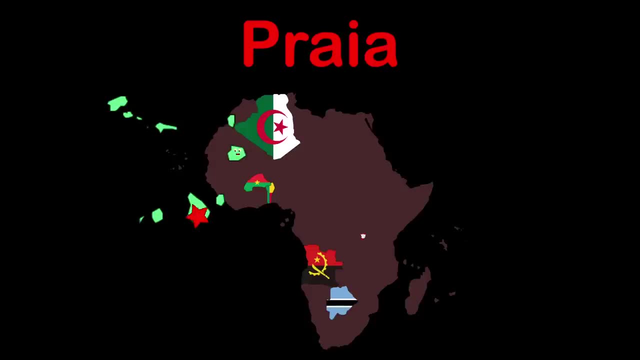 Cape Verde's my name. My capital is Raya. Come to Cameroon, Yande's, my capital, to teach. ya, I'm the Central African Republic. My capital, Bundi, is what you think I am. Chad, My capital's Mujermina. I'm Comoros, Moroni's my capital, yeah. 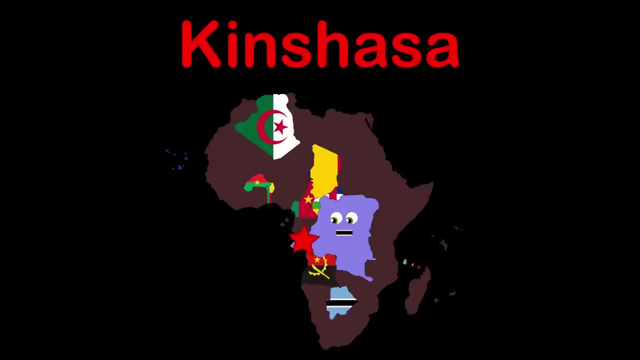 I'm the Democratic Republic of Congo, Capital's Kinshasa. I'm the Republic of the Congo, Brazil's, my capital. Cote d'Ivoire's my name Capital's Yamoussoukro. I'm Djibouti and my capital's Djibouti City. I am Egypt, Cairo's my capital and largest city. 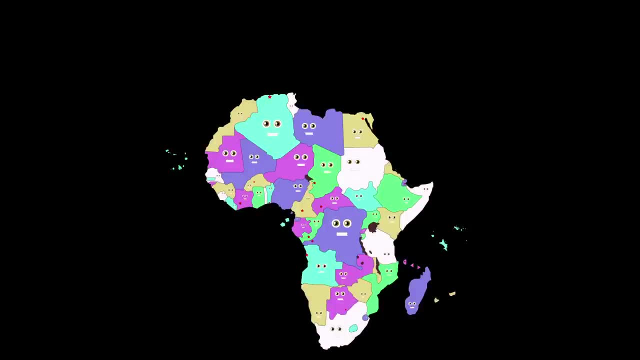 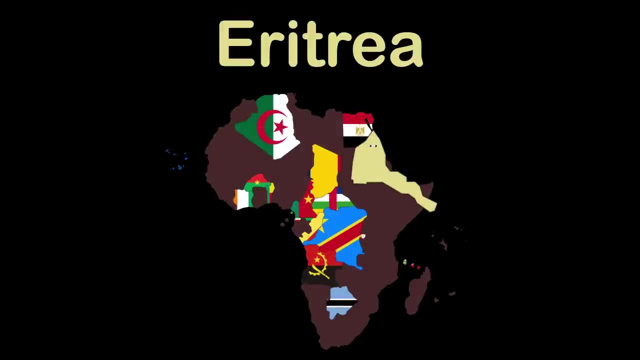 We are the countries of Africa, The planet's second largest continent, right after Asia. We are the countries of Africa. There are 54 countries presently that we will teach. ya, I'm Equatorial Guinea, Malabo's my capital. I am Eritrea, Asmara's my capital. 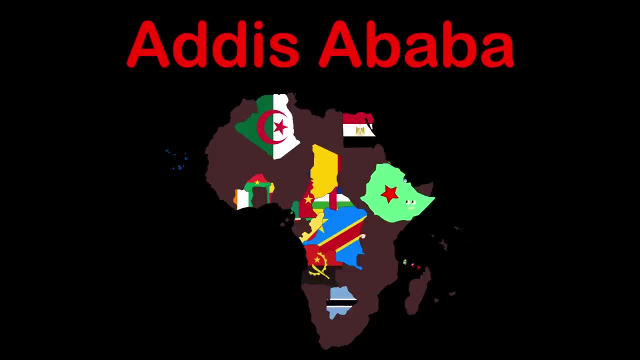 Ethiopia's my name. My capital's Addis Ababa. I'm Gabon. My capital's Lavroville, Nice, to meet. ya. My name is Gambia. My capital is Ponchou. I'm Ghana. My capital, La Croix is really cool. 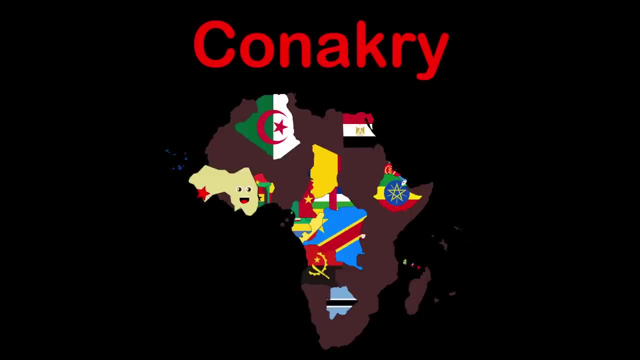 Guinea's my name, Calgary's my capital. I'm Guinea-Bissau, Bissau's my capital. My name is Kenya, My capital's, Nairobi. I'm Lesotho, My capital's, Massaroos, The place to be. 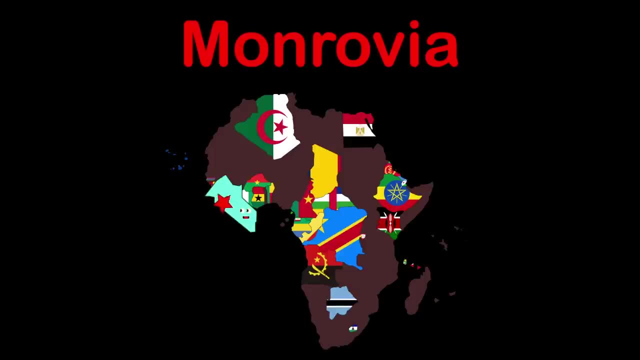 Hi. I'm Liberia. My capital's Monrovia. I'm Libya. My capital's Tripoli. in North Africa, Madagascar's my name. I'm Tananati Evo's my capital. I'm Malawi. The Elan way's really peaceful. 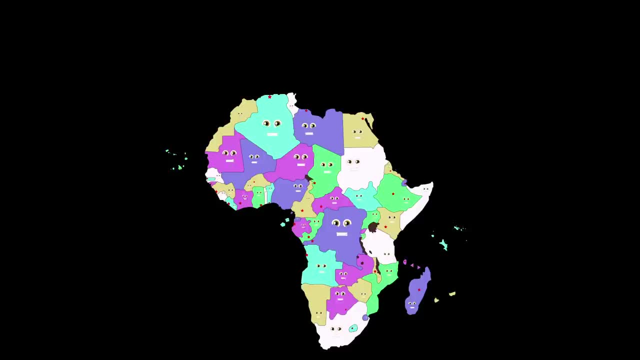 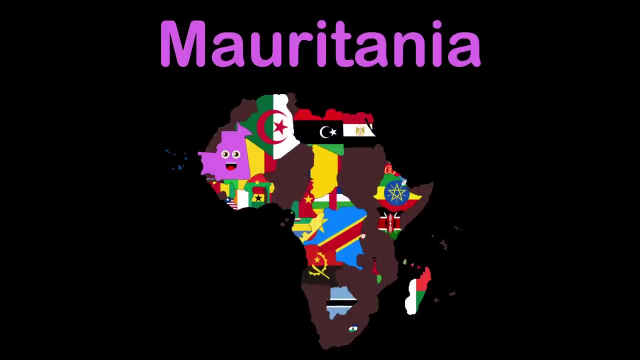 We are the countries of Africa, The planet's second largest continent, right after Asia. We are the countries of Africa. There are 54 countries presently. that we will teach ya. My name's Mali. My capital, Bamako's really hot. I'm Mauritania. My capital is now Oshad. 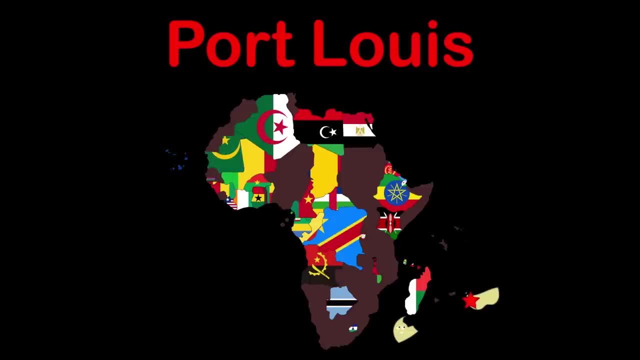 My name's Mauritius. My capital's Port Louis, How's that? I am Morocco. My capital's name is Rabat. Mozambique is my name. My capital is Maputo. I am Namibia, Windhoek's my capital. 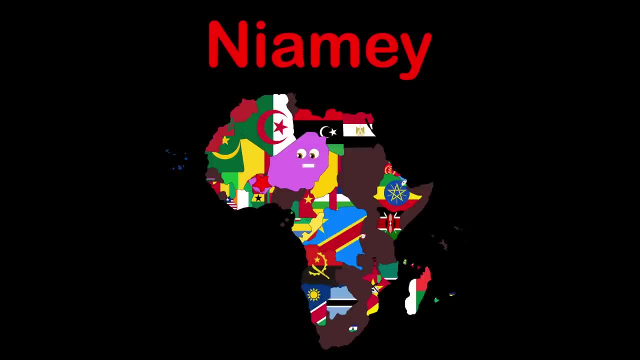 Nigeria's my name. My capital is Niamey. I am Nigeria. My capital's Abuja. here to stay. I'm Rwanda, It's me. My capital is Kigali. I'm Sao Tome and Prisipi, My capital's Sao Tome. 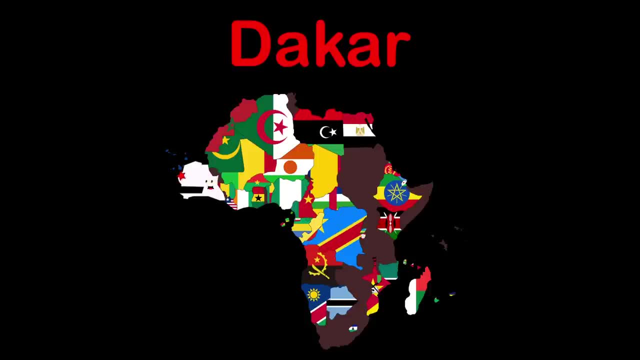 Senegal's my name. My capital is Kigali. My capital is Dakar. I am Seychelles, My capital's Victoria. My name's Seattle, My capital's Freetown, Mesilla. I'm Somalia, My capital's Mogadishu. 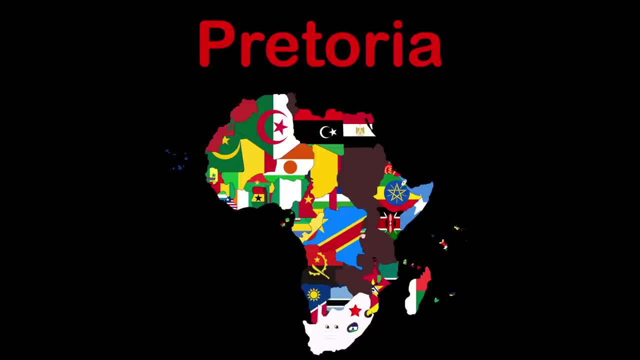 I'm South Africa, My ministry's New Capital's Pretoria. South Sudan: My capital is Juba. South Sudan, My capital's Khartoum, Now has fame. I'm Swaziland, My capital's Mbabane.